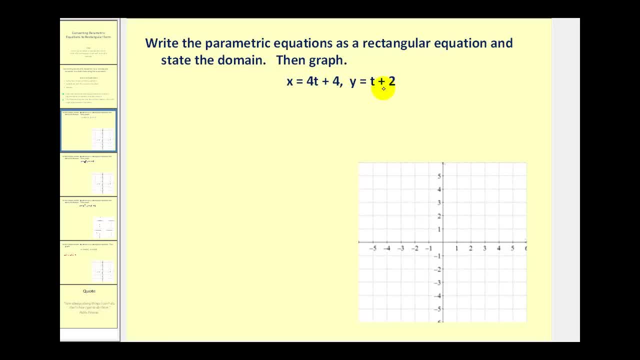 solve one of the equations for t. It's going to be easier if we solve the second equation for t. So we would have y minus two equals t. So now we'll use this to perform substitution into the first equation, where we have x equals four, t plus four. We're going to replace 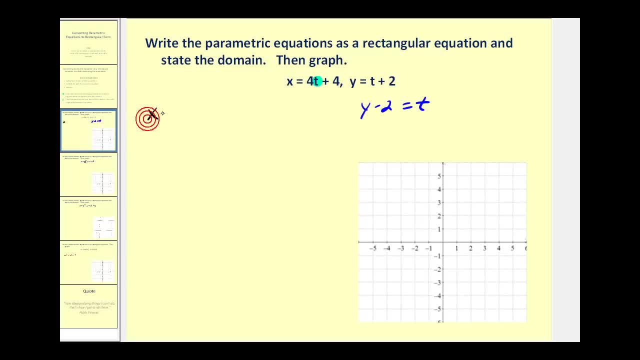 t with y minus two, So we'll have: x equals four times the quantity y minus two plus four. Now we'll simplify this and solve for y, So we'll distribute. We'll go ahead and combine our like terms. Now we'll add four to both sides, So we have x plus four. 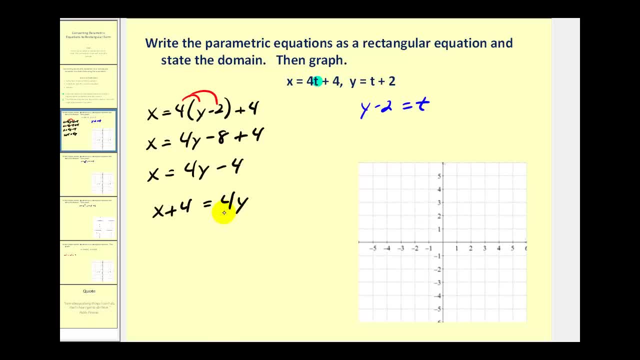 equals four y. And the last step to solve for y, we'll divide everything by four. So we would have y equals. this would be one-fourth x plus one. So these parametric equations represent a line and in rectangular form that line is: y equals one-fourth x plus one. 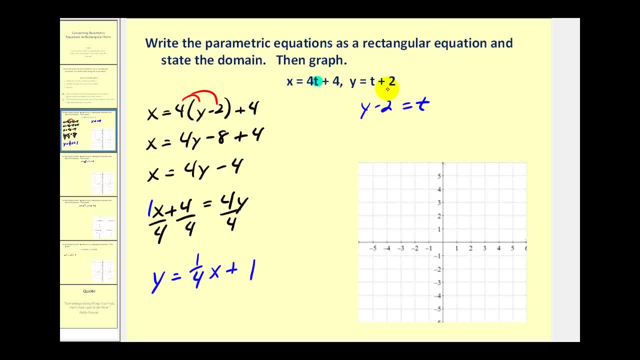 Again, notice there were no restrictions on t, So t could be any real number and therefore there's no restrictions on the domain of this line. So we can go ahead and just graph. the line y equals one-fourth x plus one, Where the y intercept is positive one and our slope is one-fourth. 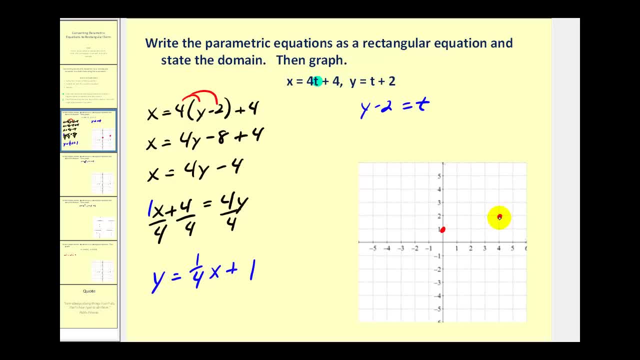 So we'll go up one right four. So our line passes through these points. Let's go and take a look at another example. Here we have: x equals the square root of t and y equals t minus five. Now, even though the restriction is not given, we know that. 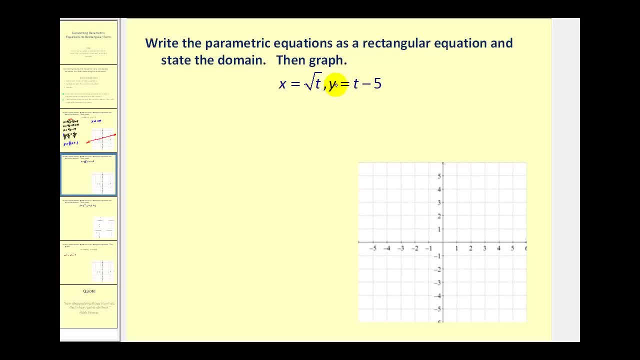 t can never be negative because we have: x equals the square root of t, So t has to be greater than or equal to zero for these parametric equations. Next, let's go ahead and solve one of these equations for t. Let's use the first equation this time, If x equals the square root of. 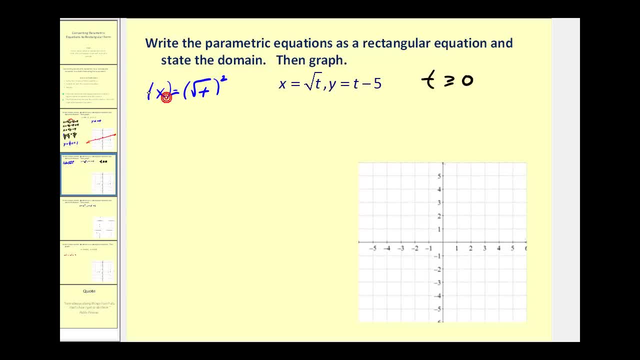 t. we could square both sides of this equation, So we'd have t equals one-fourth x plus one. So we'd have t equals one-fourth x plus one. So we'd have t equals x squared. And now we'll perform substitution. 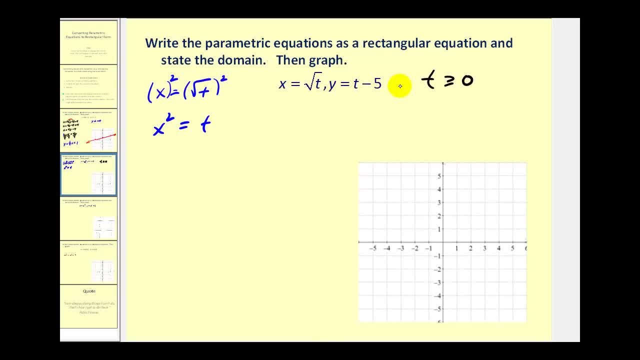 into the second equation where we have y equals t minus five. So we'll have y equals and then t is x squared minus five. So the rectangular equation is y equals x squared minus five. But since t has to be greater than or equal to zero, 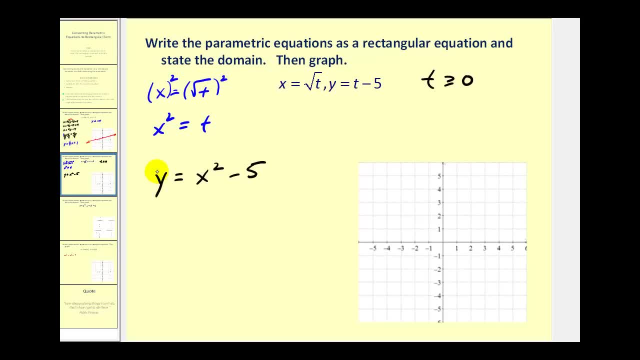 that means x will also always be greater than or equal to zero. So the domain for this function must be restricted where x is always greater than or equal to zero. So this is a parabola shifted down five units, but we're only going to graph the part when x is greater than or equal to zero. 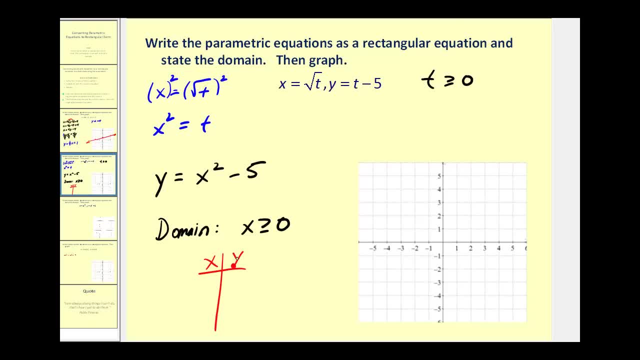 So let's go ahead and make a quick t table here. When x is zero, y would be negative five. When x is one, we'd have: y equals negative four. When x is two, we'd have four minus five, That'd be negative one. 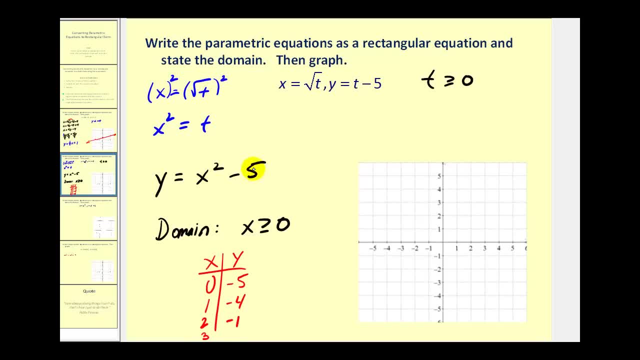 And lastly, when x is three nine minus five, That would give us y equals four. Let's go ahead and plot these points. Here's: zero negative five, one negative four, two negative one and three four. This would be the graph. 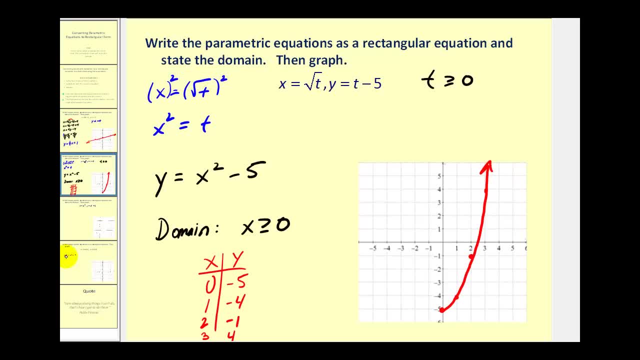 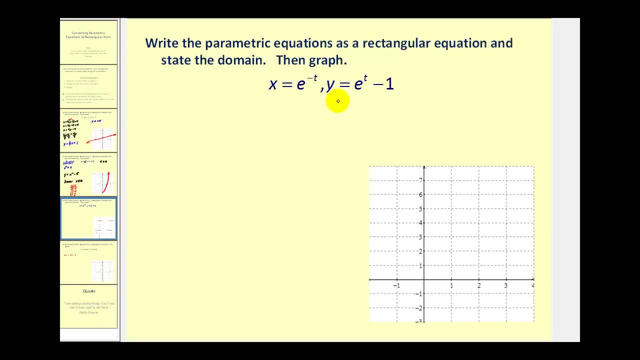 of our curve. Let's take a look at two more examples. Here we have x equals e to the negative t and y equals e to the t minus one. These are going to be a little bit more challenging to solve for t, but let's go ahead and try to solve this first. 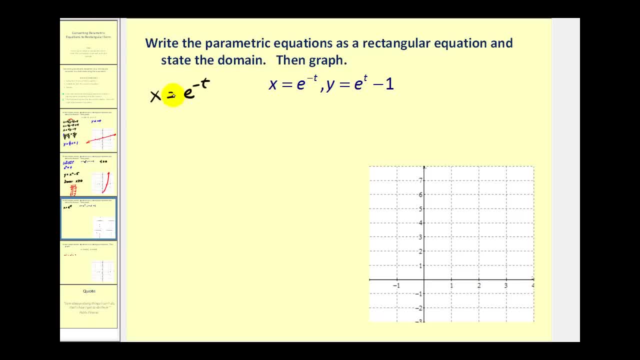 equation for t. The way we're going to do this is rewrite this exponential equation as a log equation. So let's go ahead and review this for a minute. Remember, if we have e raised to the power of b equals a. it's also true that natural log a is equal to b. 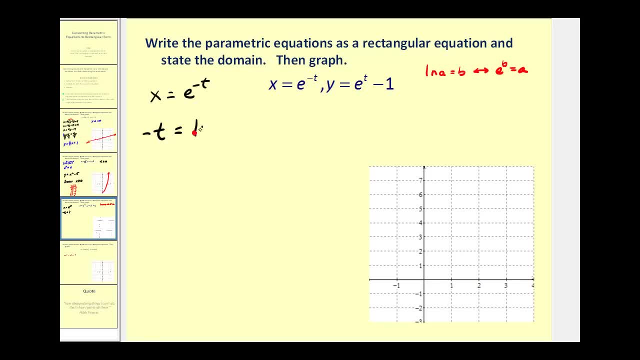 So in this case we'd have the exponent negative. t must equal natural log x. So if we were to solve this equation for t, we'd multiply both sides by negative one. We'd have t equals negative one times natural log x. And now we'll take advantage of the power. 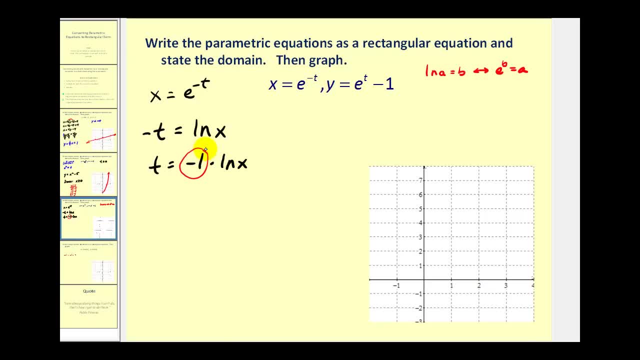 property of logs, which means we can take this coefficient and move it to the exponent on the x. So we have t equals natural log x raised to the power of negative one. And now we'll take this and perform substitution into the second equation, when y is equal to e, to the t. 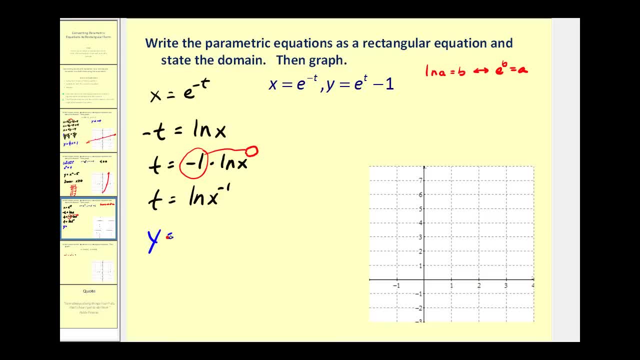 minus one, So we have y equals e to the natural log, x to the power of negative one minus one. And now we'll take advantage of another property of logarithms. Remember: if this base and the base of the log are equal, this is just going to give us x to the negative one, So we'll have y equals. 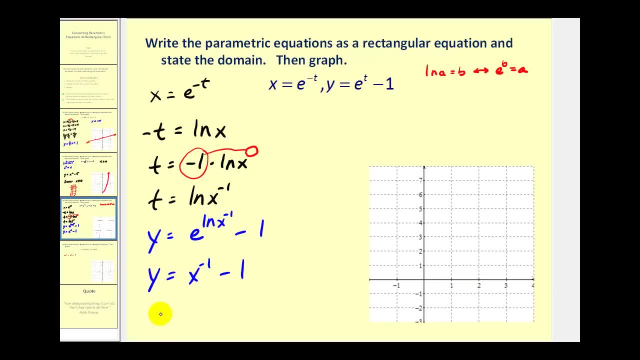 x to the negative, one minus one, which is the same as y equals one over x minus one. Now let's talk about the domain for a minute. Notice: there were no restrictions on t in the original parametric equations, Meaning t could be any real number. 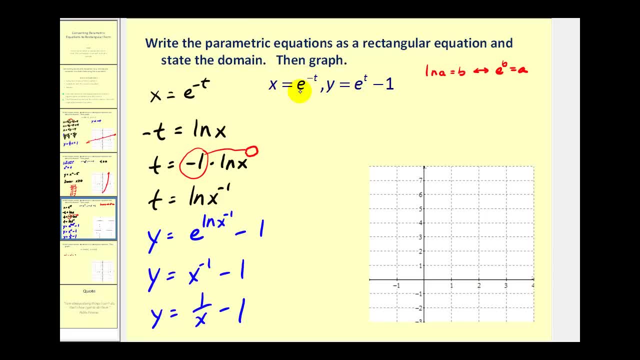 But notice that t is also the exponent on e. So in both cases here, if we take e and raise it to the power of negative t or positive t, it's always going to be greater than zero. So if e to the negative t is always 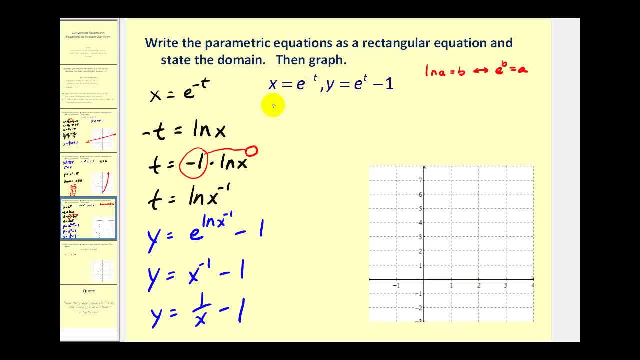 greater than zero, x is also always going to be greater than zero. Therefore, we do have to restrict the domain to x being greater than zero. So let's go ahead and make a t table for this graph, But only select values when x is greater than zero. 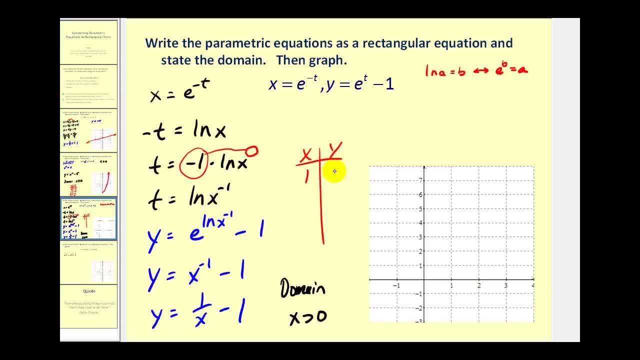 So if x is equal to one, we'd have one minus one. that would be zero. When x is equal to two, we'll have one half minus one. that would be negative one half. Let's go ahead and select: x equals one half. 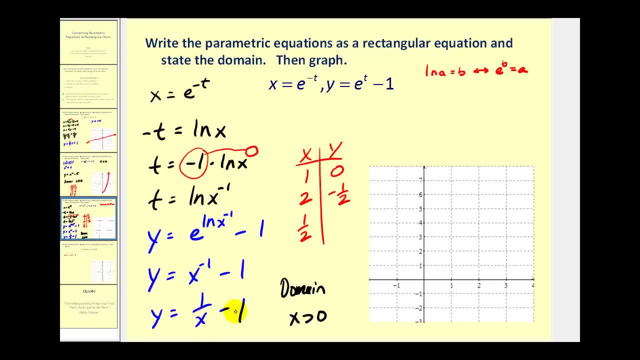 Well, one divided by one half, that's going to give us two minus one. So y is equal to one. Let's go ahead and plot these points. Here's one zero, Two negative, one half would be here And one half one would be here. 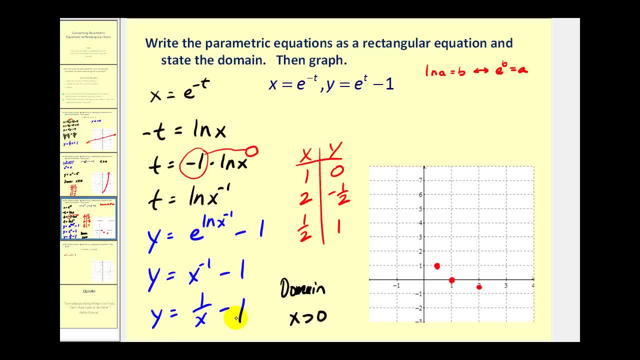 Notice, as x approaches infinity, y is going to approach negative one. So we do have a horizontal asymptote here, And we also have a vertical asymptote at x equals zero. So we have a graph that looks something like this: With our restricted domain, Let's go and take a look at one more. 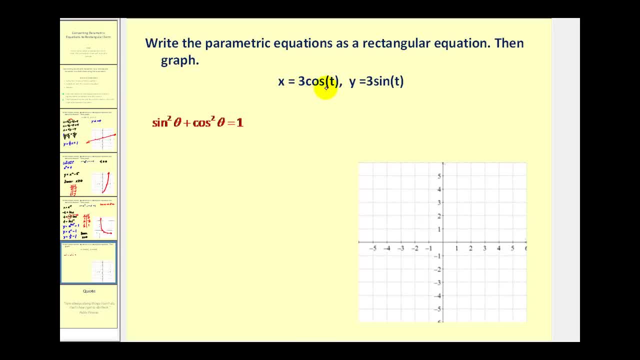 Notice on this last example. we have x equals three cosine t and y equals three sine t. Both of these involve trick functions, So in this case we'll use the identity sine squared theta plus cosine squared theta equals one to eliminate the variable t. 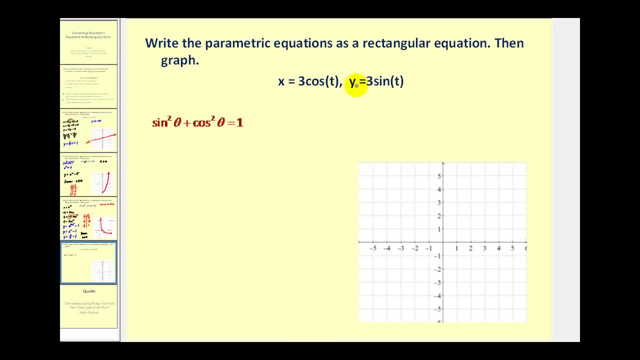 The way we'll do that is, we'll solve this first equation for cosine t and then we'll solve the second equation for sine t. So cosine t would be equal to x divided by three, and sine t would be equal to y divided by three. 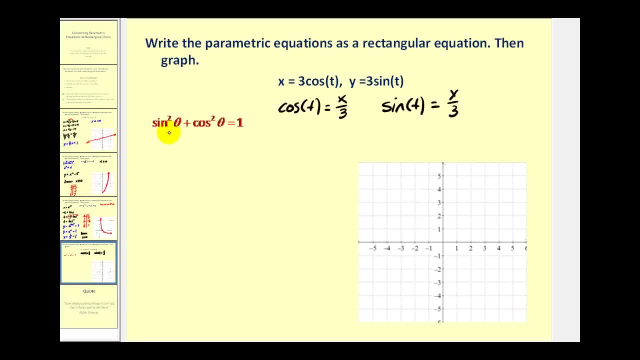 Now, using this trick identity, we can replace sine squared theta with y over three squared. And we can replace cosine squared theta with x over three squared, And this sum must also equal one based upon this identity. So now we'll go ahead and simplify. 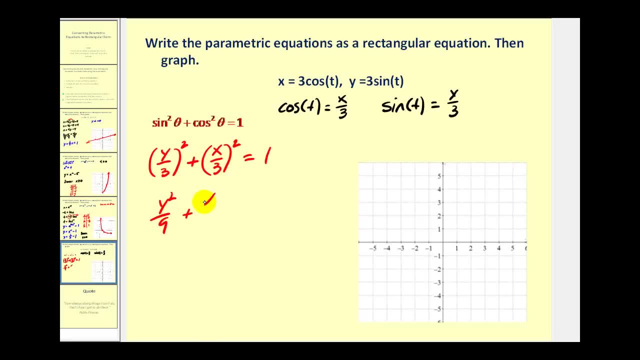 We'd have: y squared over nine Plus x squared over nine equals one. Now we'll multiply everything by nine, So we'll have y squared plus x squared equals nine. Now we should begin to recognize this as a circle Where the center is at zero zero and the radius is equal to three. 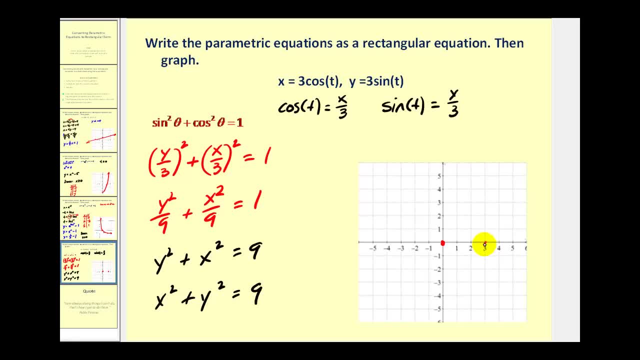 So here's the center, And since the radius is equal to three, we'll plot four points out, three units from the center, And now we can sketch the circle, And there it is. Okay, that's going to do it for this video. I hope you found this helpful. 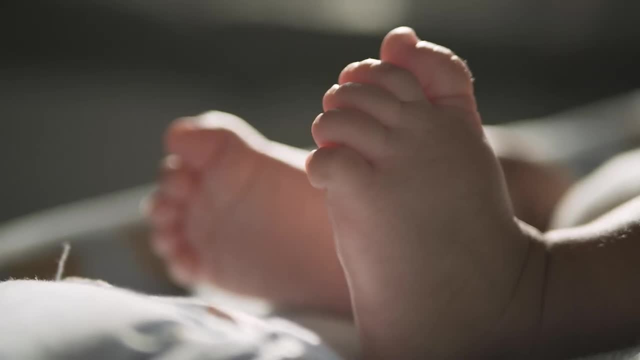 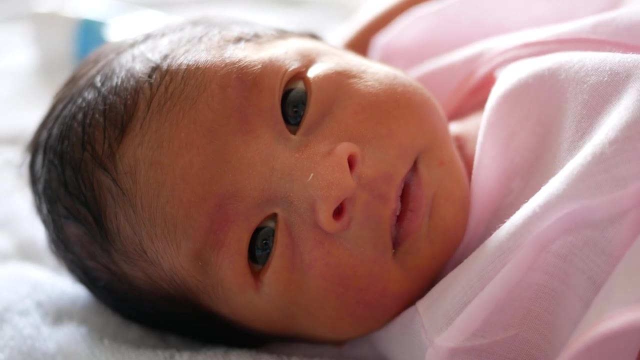 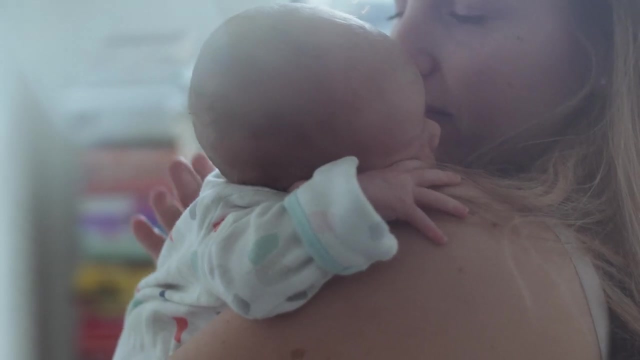 On your family's biggest day. at Christus Health, we deliver the little moments: From the first time holding your baby, sparking that initial bond, to the attentive care during a late night feeding, to the reassurance our Level 3 NICU brings. every miracle deserves its moment.